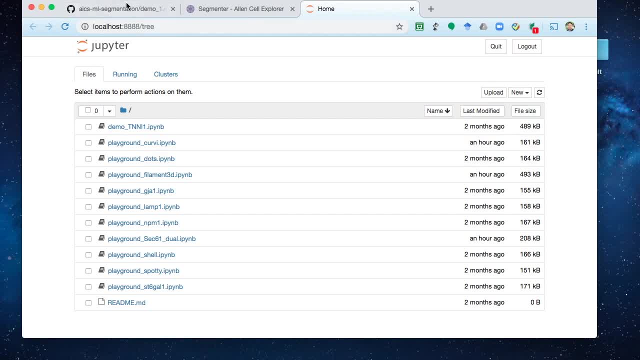 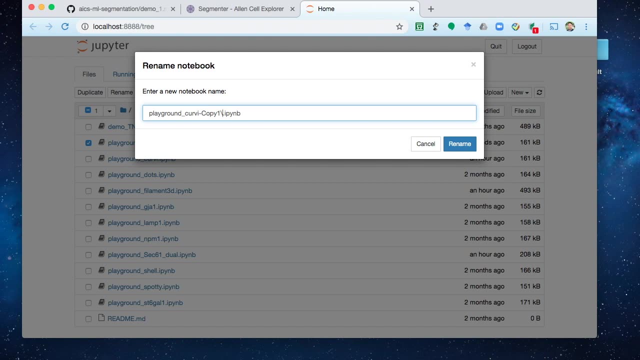 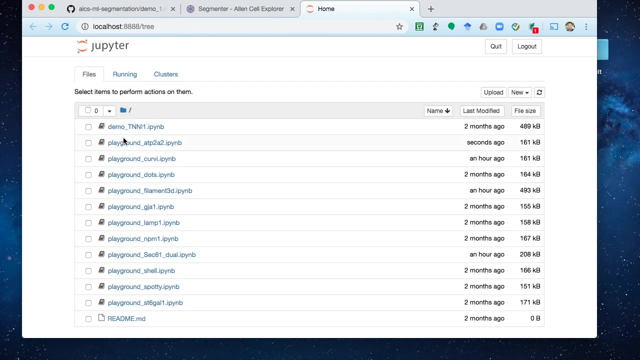 For example, we'll copy the input of atp-218 through a index. We'll make a copy of the notebook containing workflows for sex 61-beta And rename the notebook accordingly to ATP-282.. We're now ready to create a segmentation workflow for ATP-282.. 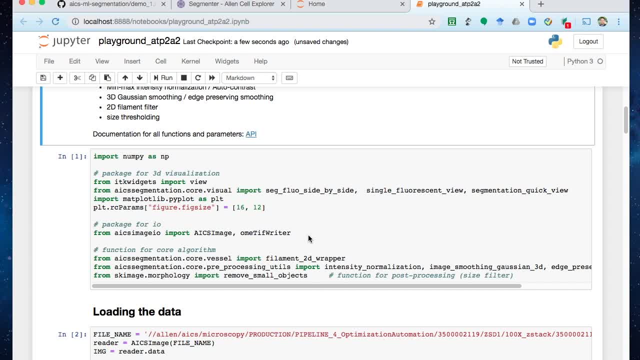 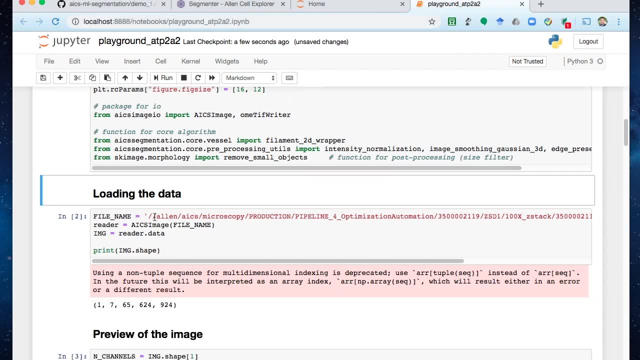 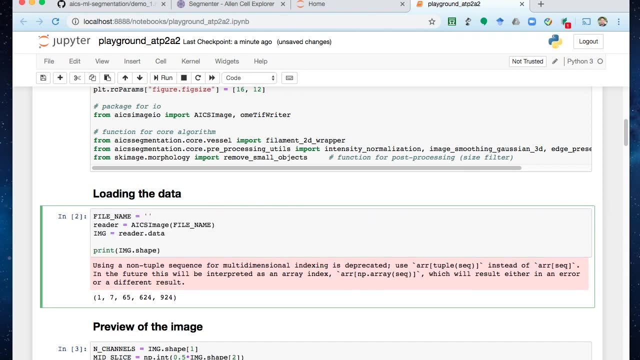 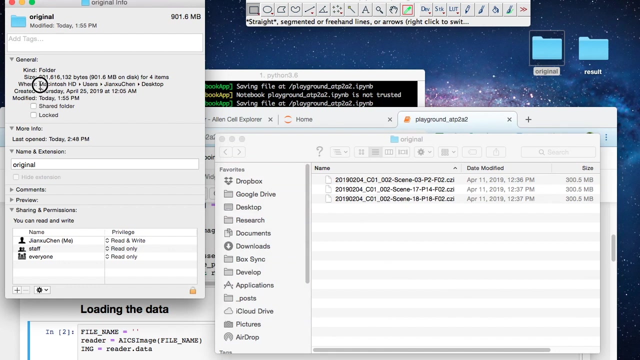 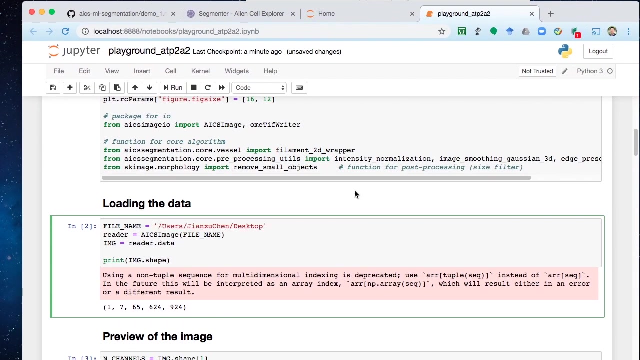 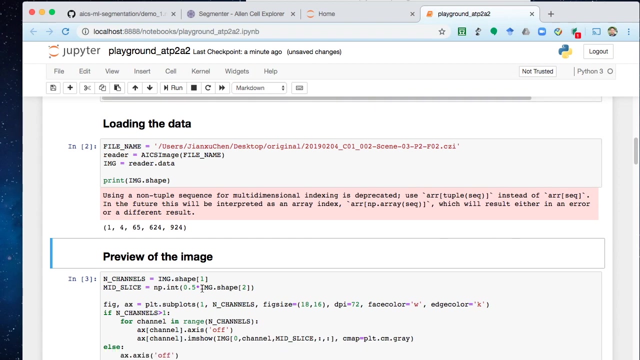 First we import the necessary packages, and then we'll need to load an image. All you need to do here is to find the file path of the image you would like to work on and copy-paste it to the notebook. We can then preview the image and notice that this image has four channels. 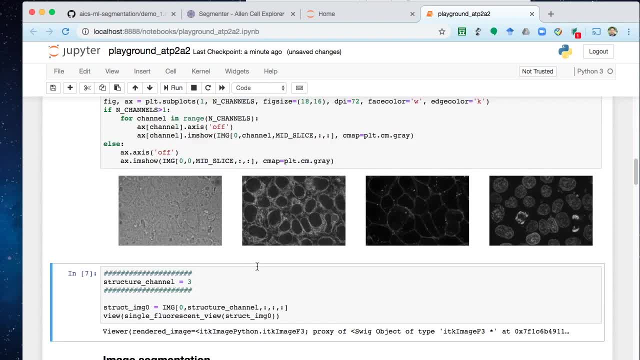 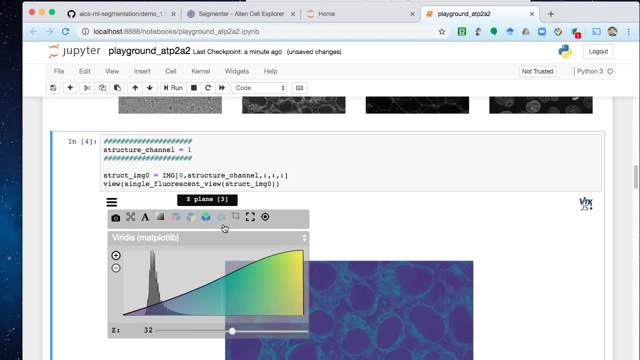 The channel containing the structure is the second one, But since Python uses zero-based indexing, we'll need to change the structure channel to 1.. Once you specify the image channel, you can take a look using this tool. Let's take a look on this built-in ITK viewer. 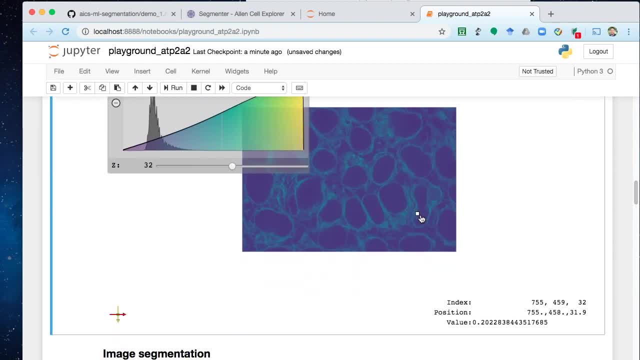 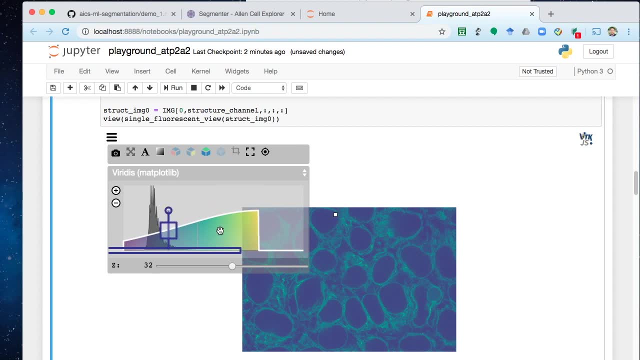 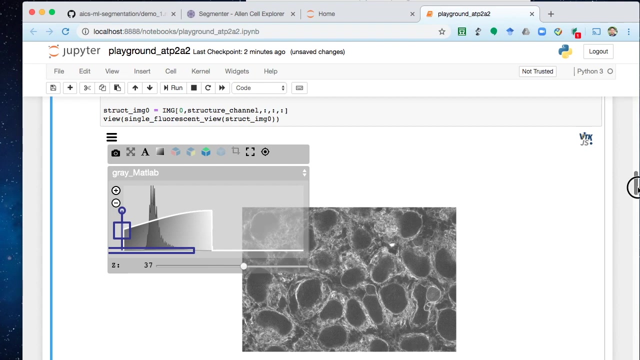 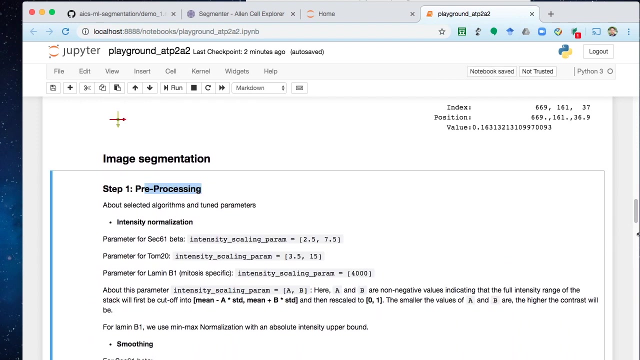 The viewer allows you to adjust image contrast, going up and down through z-slices, as well as adjusting the color map. Now we know what the image looks like, we're moving on to the pre-processing part of the workflow. The first part is to normalize the intensity so that the structure won't be too dim. 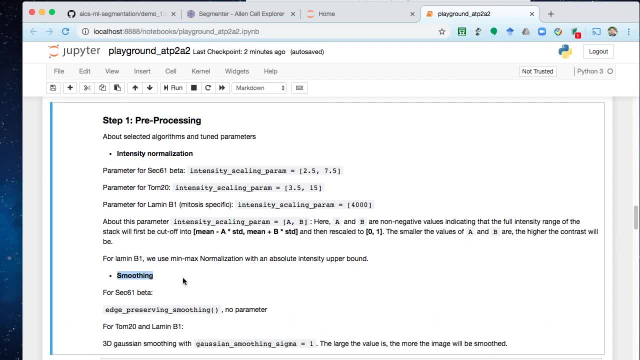 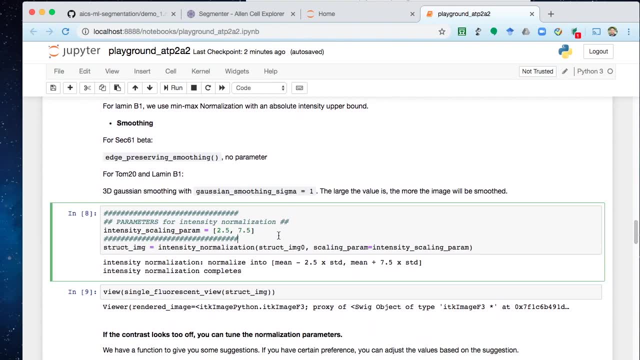 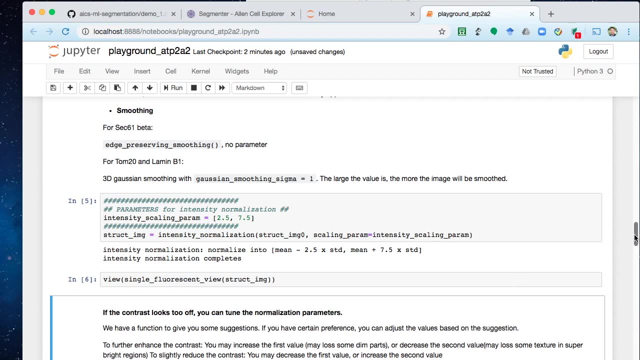 Also, the normalization can help make multiple images more consistent for batch processing and the following segmentation steps more robust. Here we'll try the default parameters at sec61-beta. You can adjust the contrast based on instructions in Python. You can adjust the contrast based on instructions embedded in the notebook, if needed. 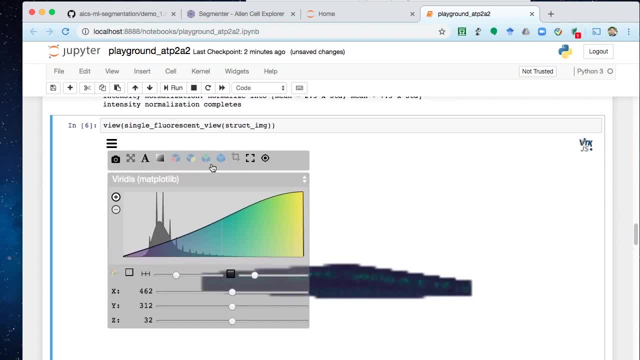 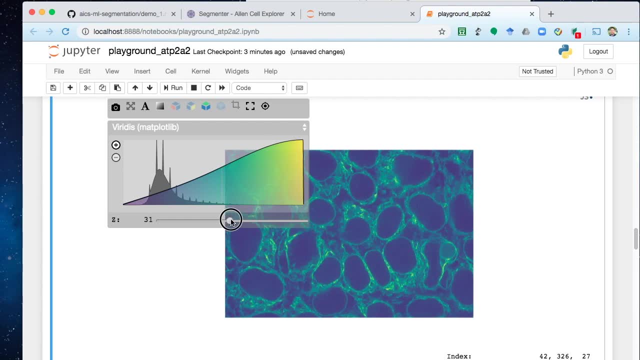 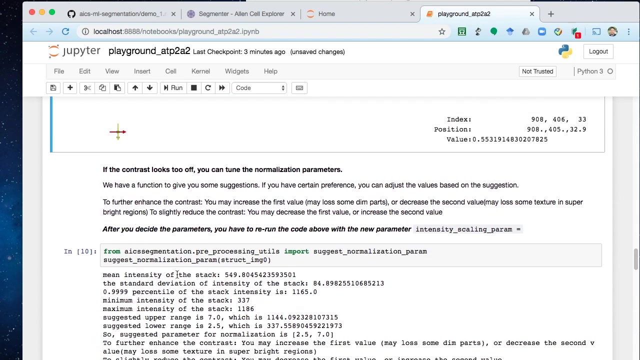 As this tutorial mainly focuses on how to use the segmenter, we'll leave out the question about if the adjusted image looks good or not. You can decide that for your own data. Next we'll do smoothing- Nothing to change here in the code. 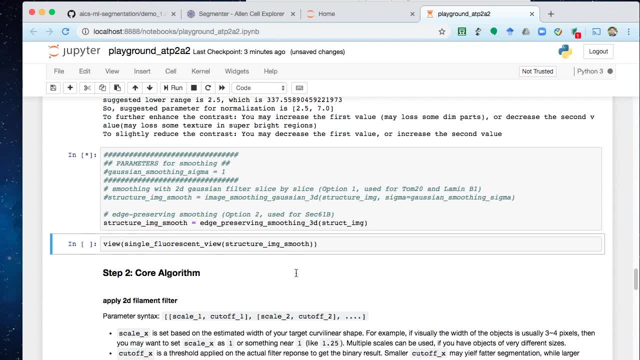 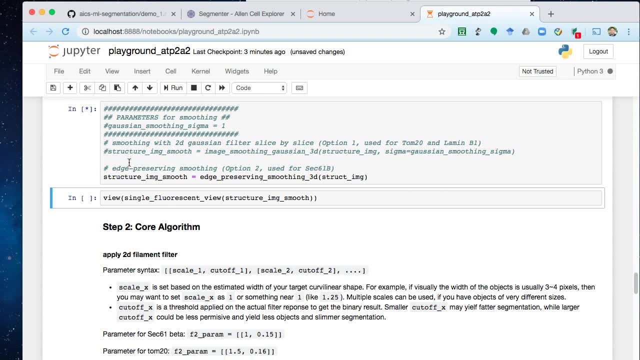 If you're not familiar with Jupyter, having a star next to the block means that the code is running. Sometimes this can take a minute. I wanna give you a quick demonstration. The first thing we'll do is to run it again. 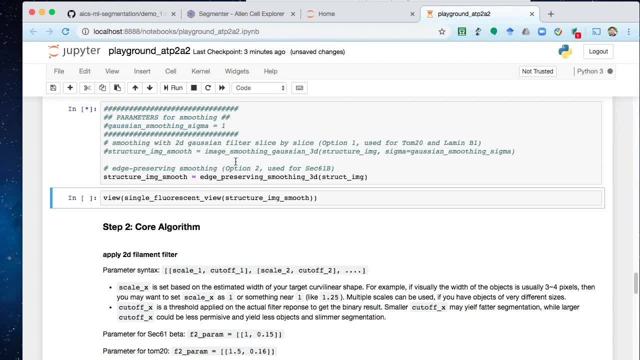 You can see that the code is running. You can use a back-of-the-box example to take a look at how smooth the image can be. As you can see, it's running. The blue line means that the code is damaged. Don't worry. 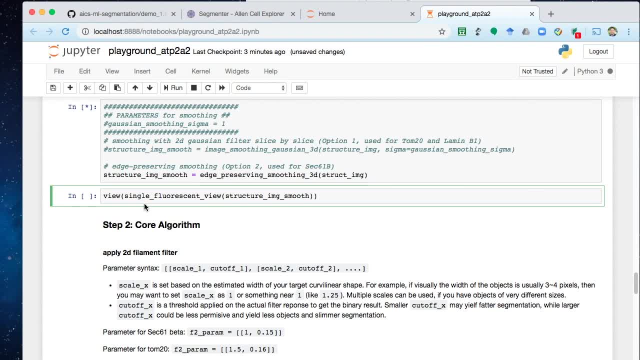 it's being the same for all the other pieces here. The same for the other pieces. Once the code is done running, you can use the Viewer to see the smoothed image. This is the back-of-the-box example. If you want to see theunuble image. 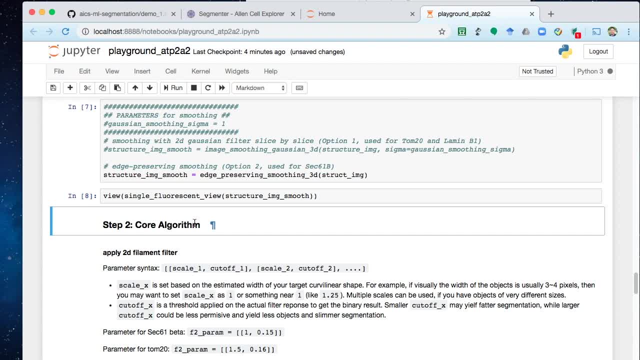 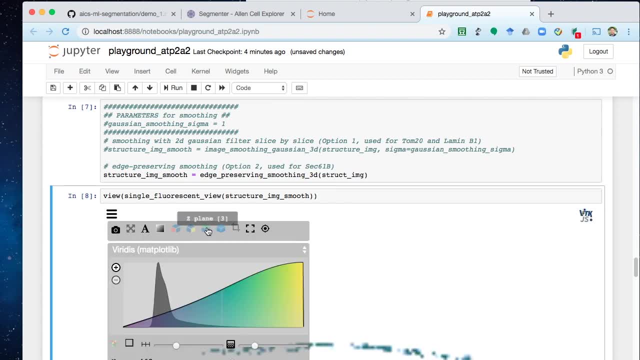 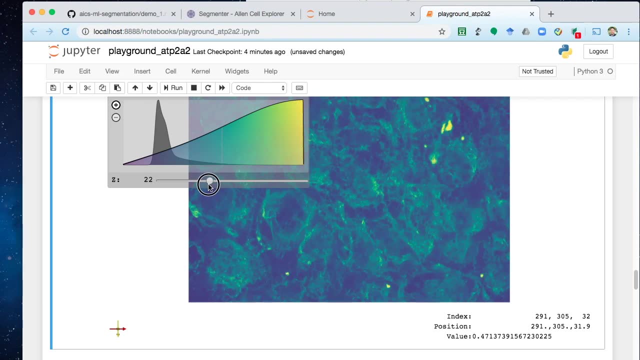 you can use the Viewer to see its smoothed image. The back-of-the-box example is still running. Once the code is done running, you can use the Viewer to see the smoothed image. The pre-processed image looks good to me. We can then move on to the core algorithms. 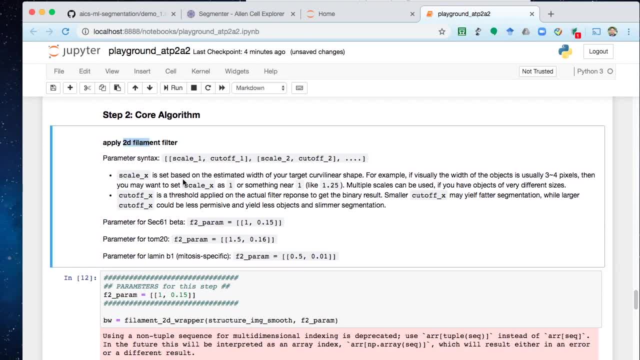 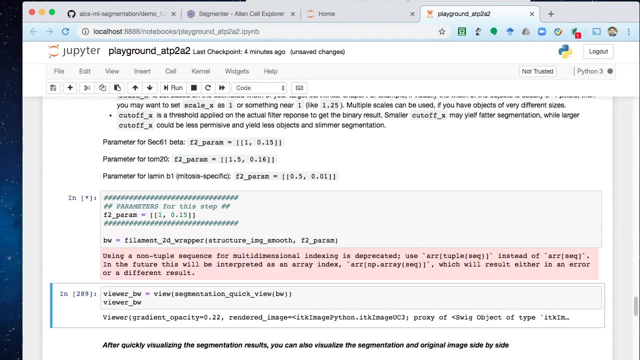 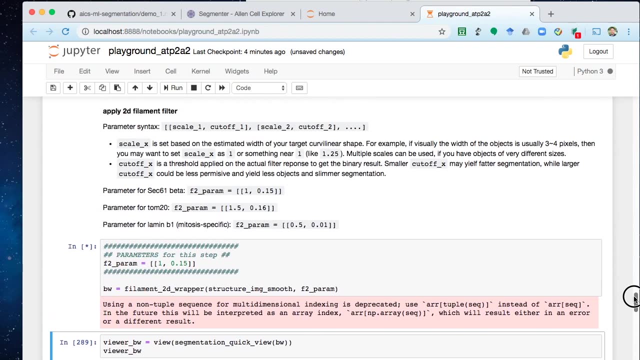 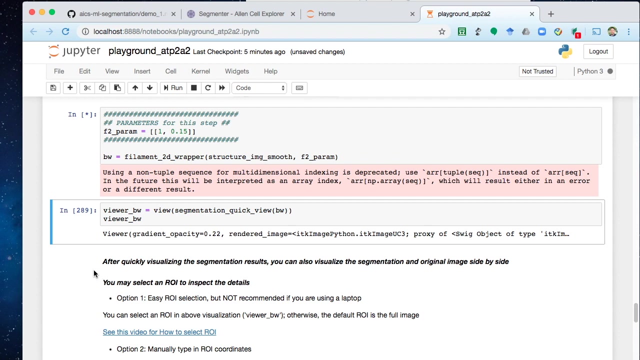 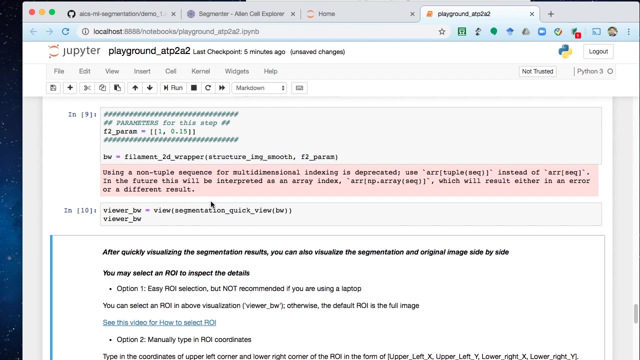 We'll set the parameters same to sec6 when beta, since the two structures look very similar. Again, the running of the code can take a minute. You can immediately view the result for segmentation here. once the code is done running, The segmentation result should be binary. 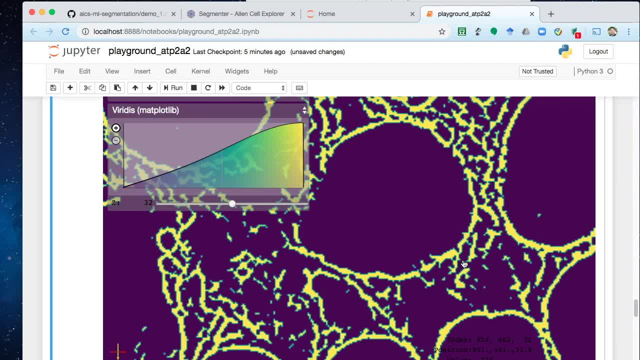 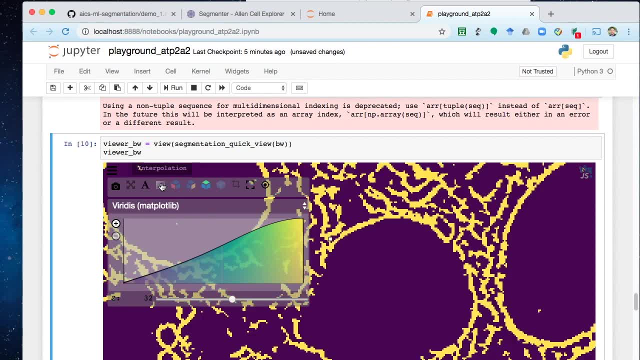 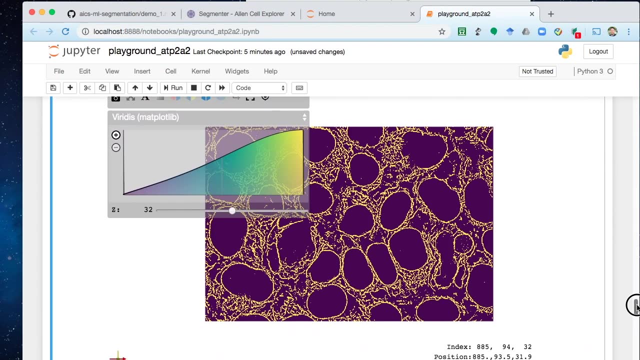 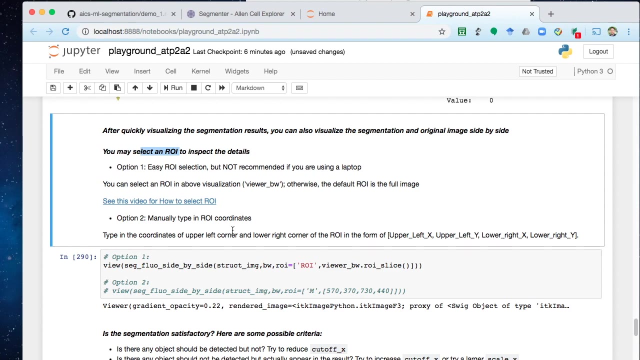 The viewer has a default setting which may smooth the edges. You can turn it off to view the actual binary result. The notebook allows you to compare the segmentation and the regional image side by side. on any region of interest You can directly select the ROI within the segmentation result. 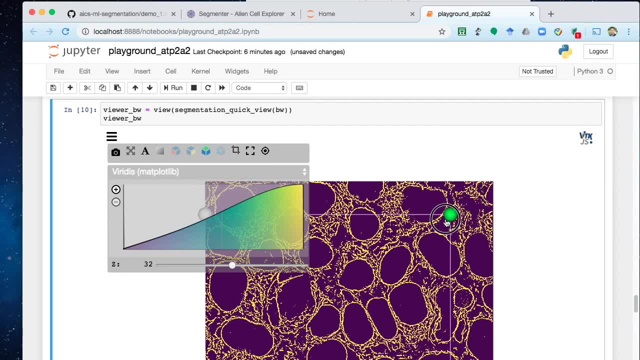 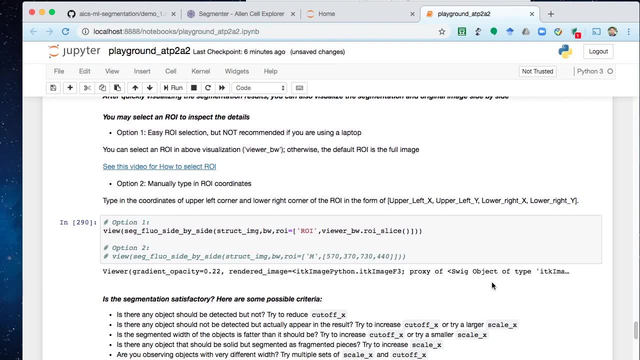 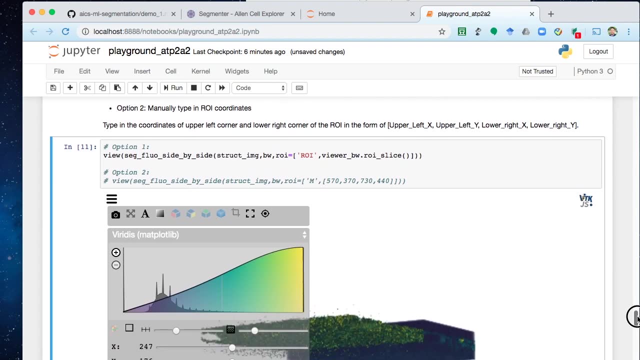 Okay, There are actually two ways to do it. We're using the first one in this tutorial, Since we noticed some instability on old computers when using option 1, we're providing a second option as backup Here. option 1 uses ROI you just used in the previous viewer and automatically loaded for. 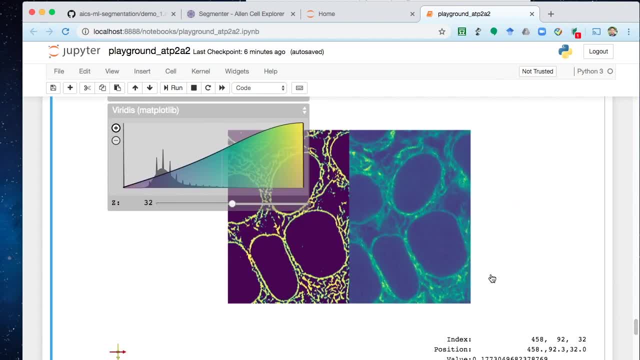 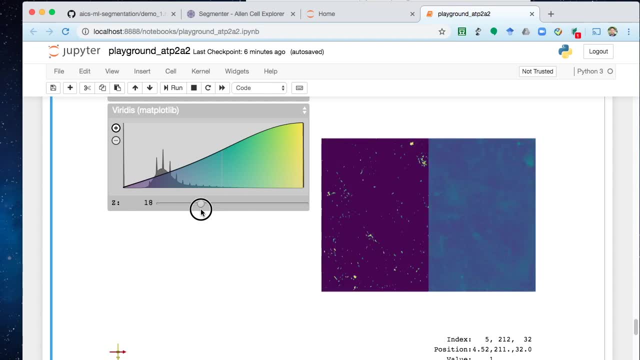 side by side comparison. We can move up and down different Z slices to look at the details. When we go to a lower Z position we can see some out of focus signals. The Z is still being picked up. Similar problem for the Z near the top. 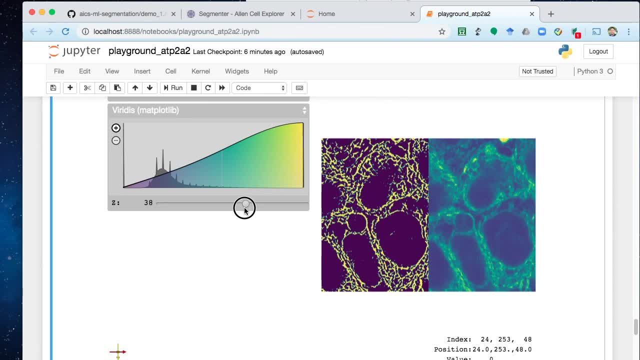 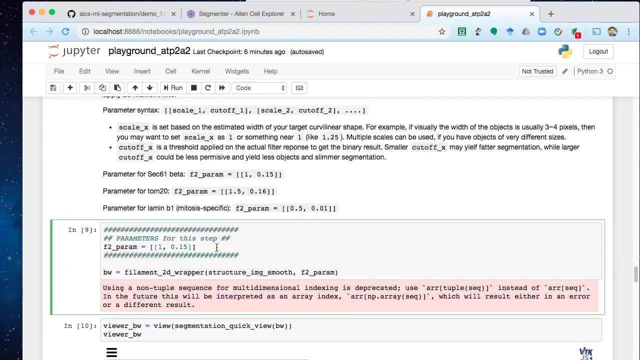 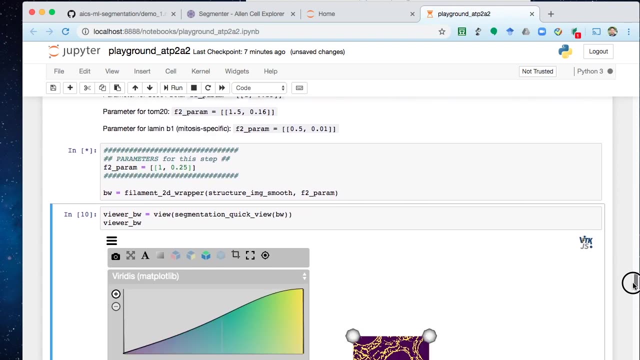 The notebook has some suggestion to deal with unsatisfactory results. In our case, we're detecting noise that should not appear in the result. We'll increase the cutoff parameter to 0.25 to make the filter less permissive and we'll run the code again. 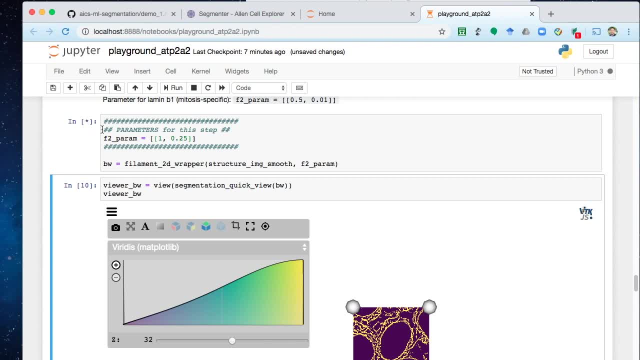 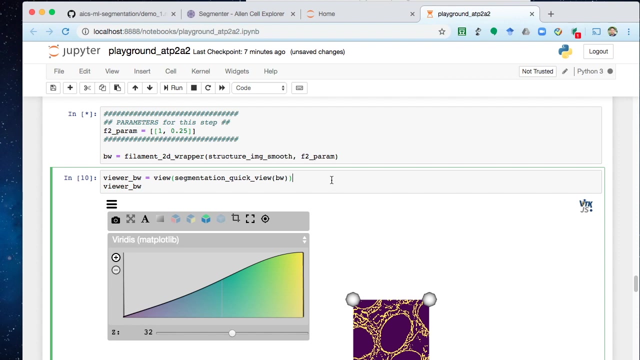 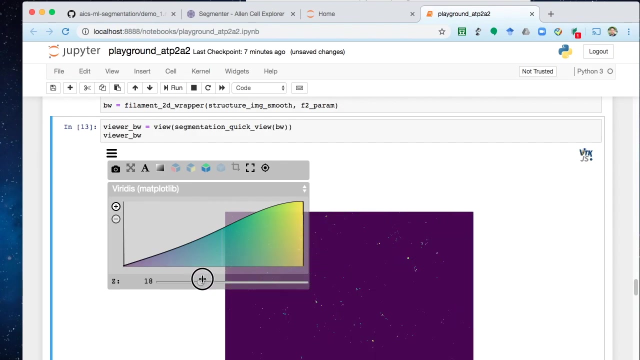 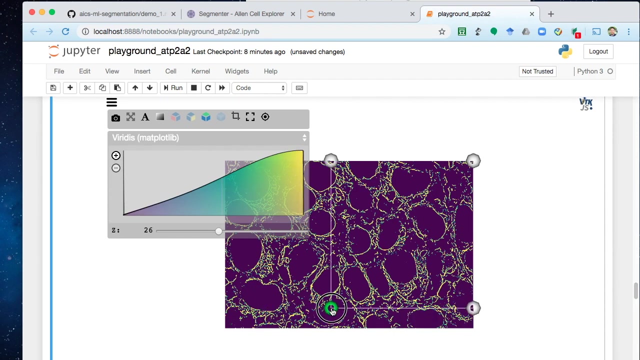 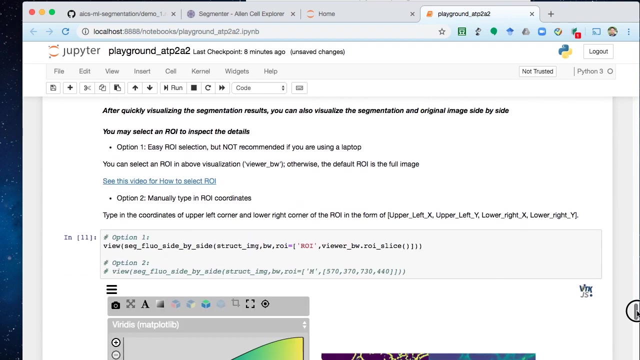 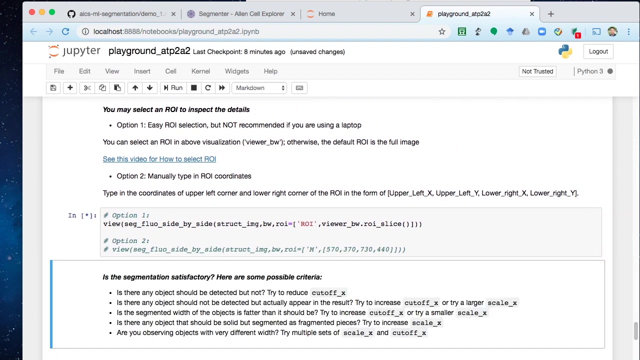 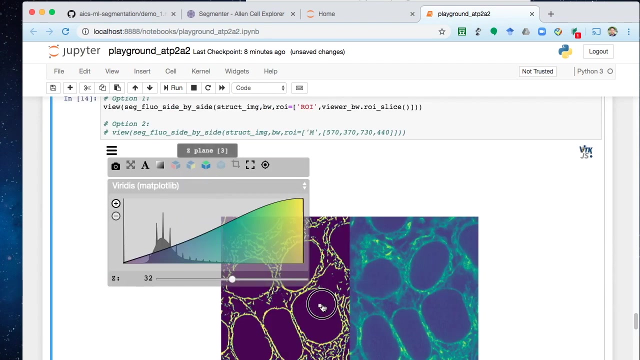 Thank you, The code is done, running and we can look at the new result using the viewer. Again, we can choose ROIs to take a closer look. This is a ROI similar to what we selected last time. We can see the result near the top and the bottom is better. 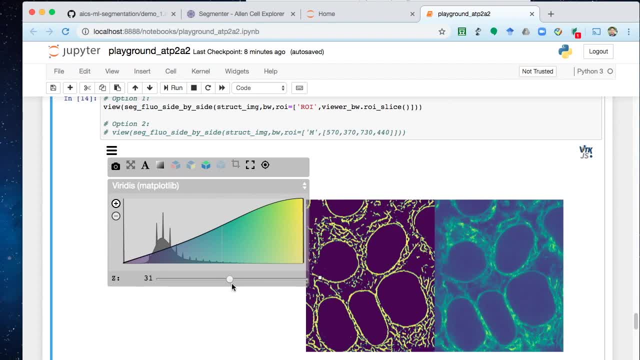 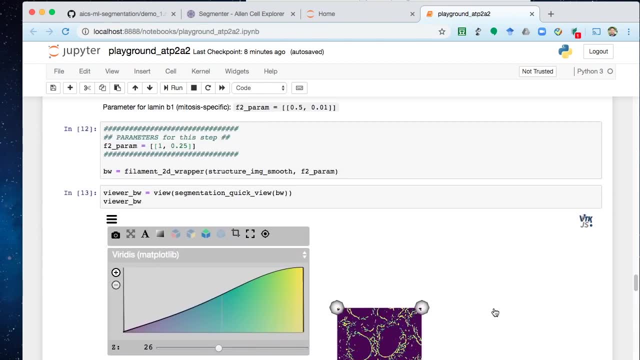 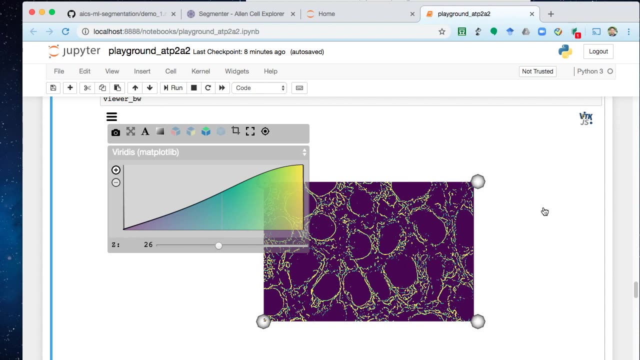 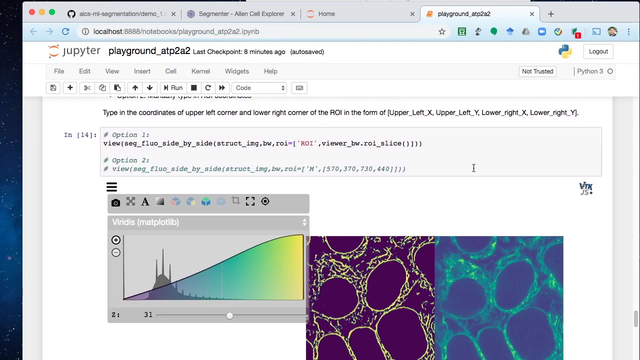 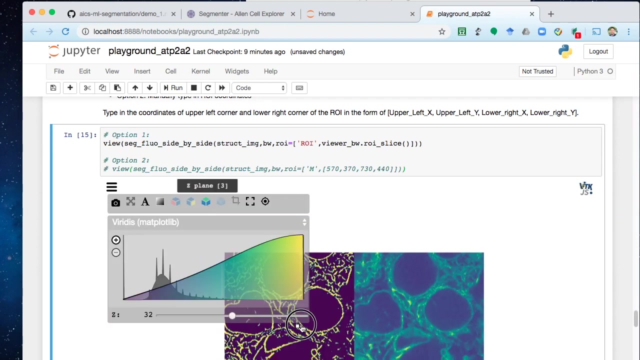 There is still some noise, but they are small enough that the post-processing step should remove them. We can also select a different ROI and it will be updated at the side-by-side view automatically. The segmentation looks pretty good Now we can see the result. 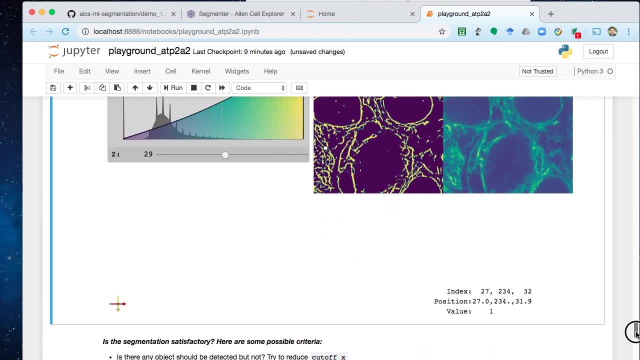 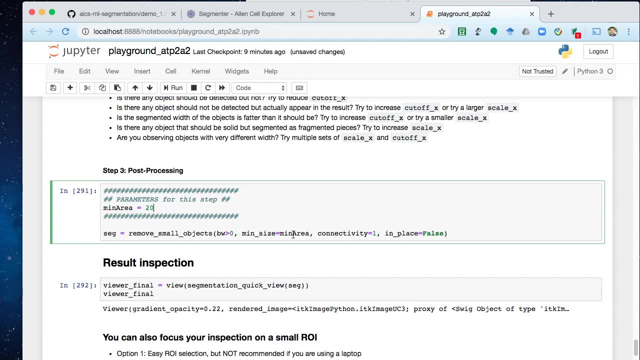 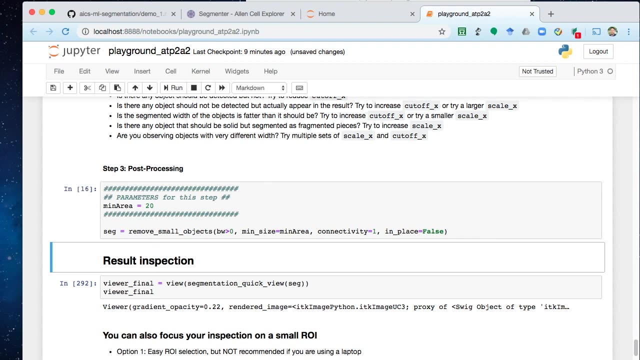 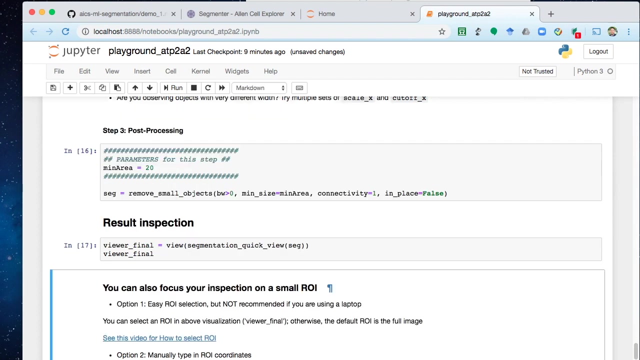 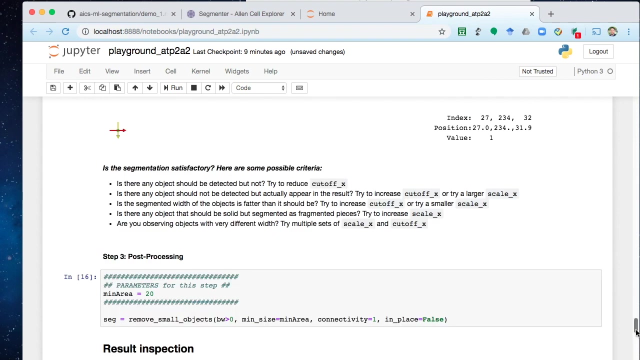 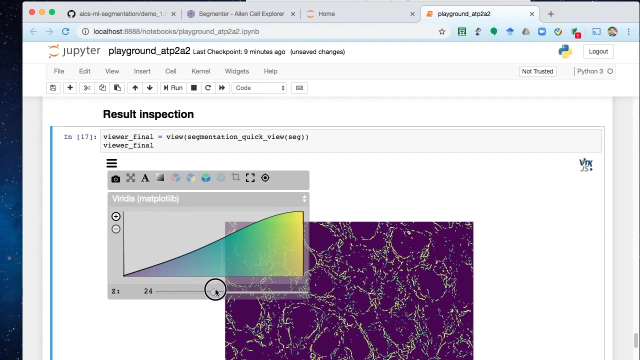 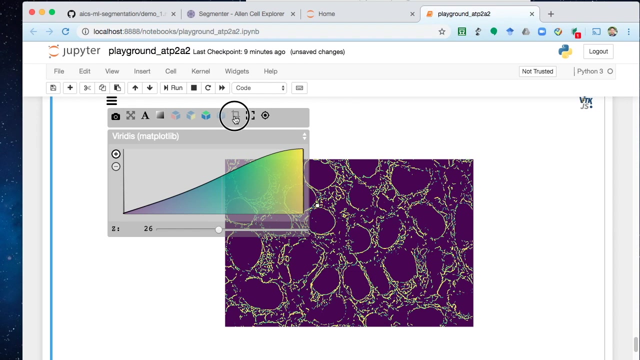 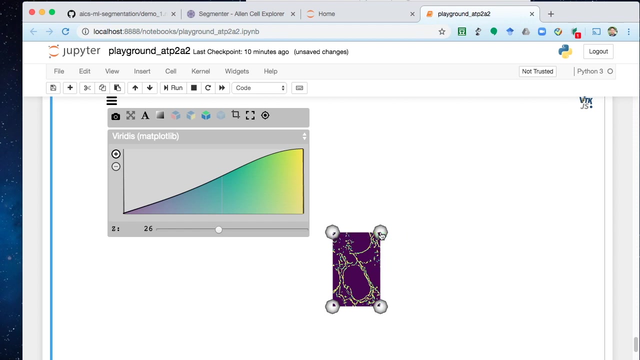 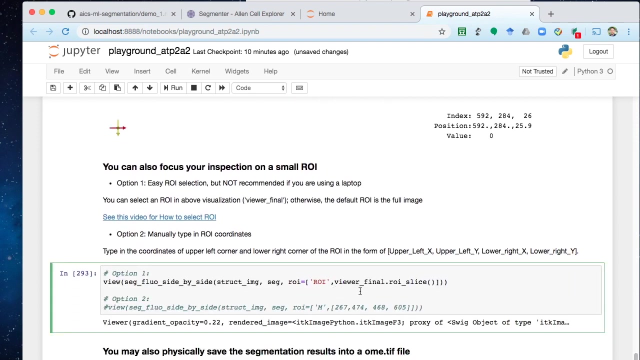 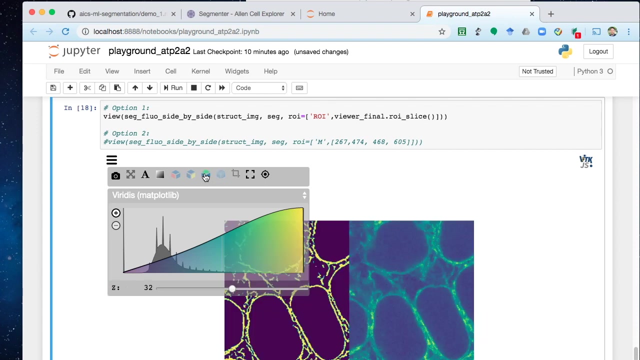 We can finish the last step, which is post-processing, to remove the small noisy spots. Here the viewer is showing the final result from the segmentation. Again, we will use the first option for comparison. This option automatically loads the ROI we selected After the final inspection. if you are happy with the segmentation result, you can export it at the end of the notebook. 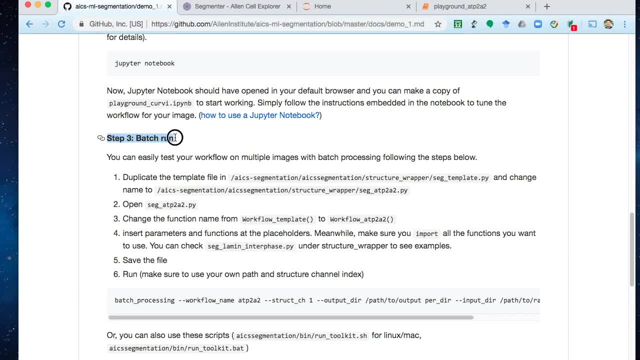 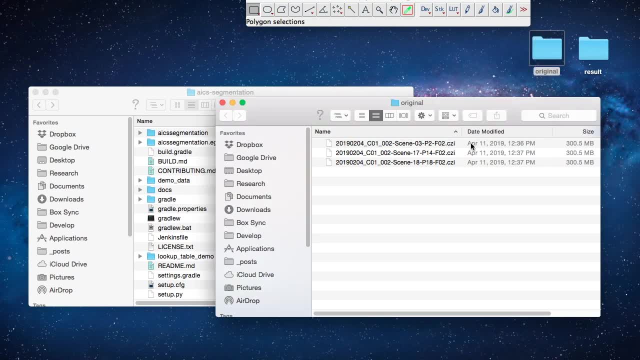 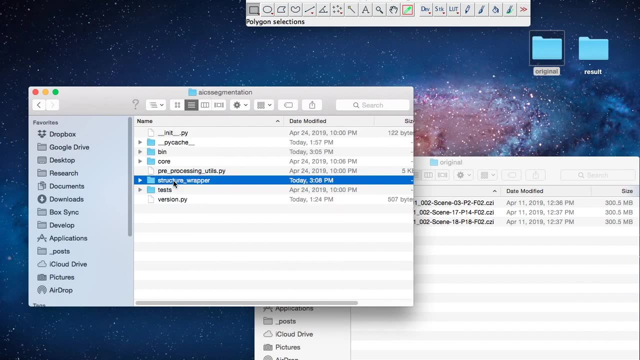 Now I will show you how to apply the workflow we set up for a single image in Jupyter Notebook to multiple ones with batch processing. Here we have a set of images we want to analyze in this demo. First we will go to the structure wrapper folder, make a copy of the template Python file. Here we have a set of images we want to analyze in this demo. First we will go to the structure wrapper folder, make a copy of the template Python file. Here we have a set of images we want to analyze in this demo. 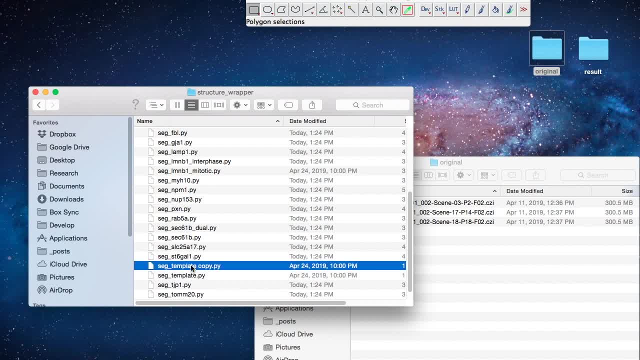 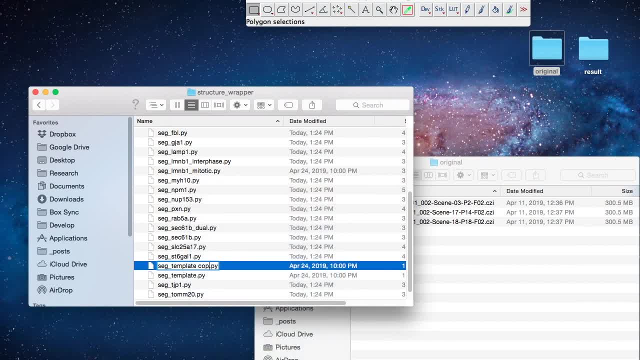 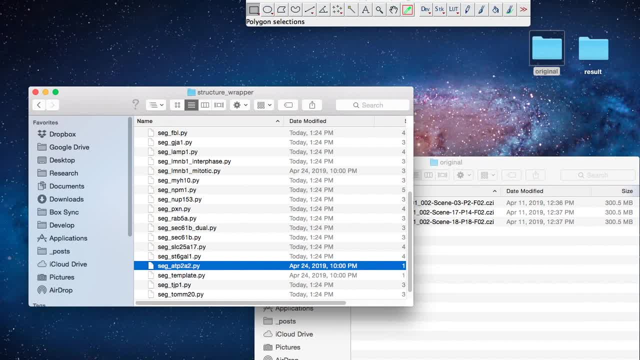 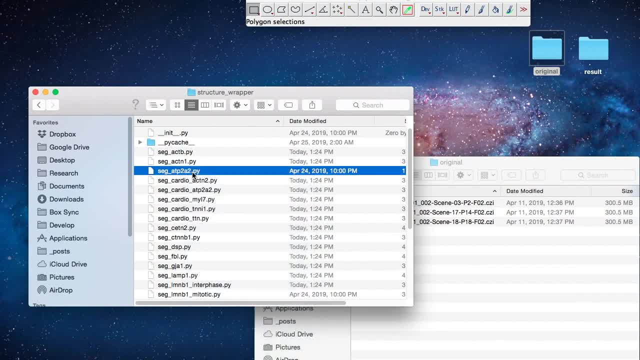 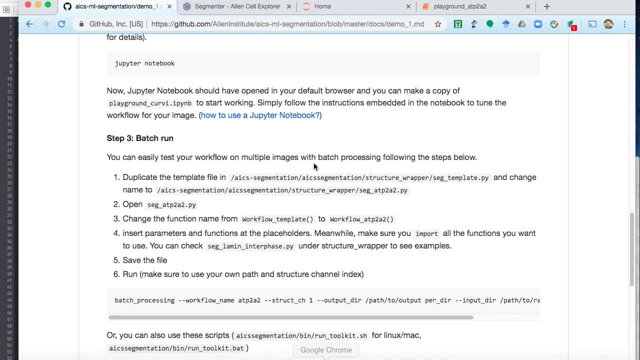 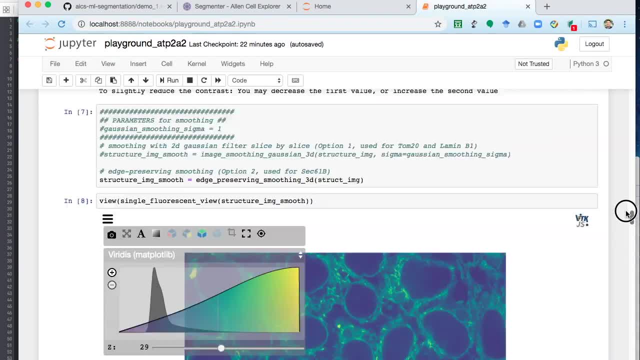 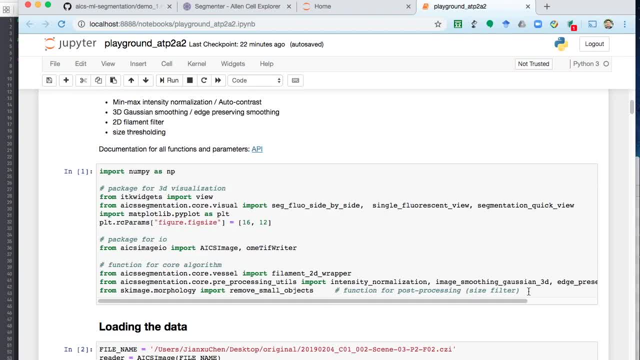 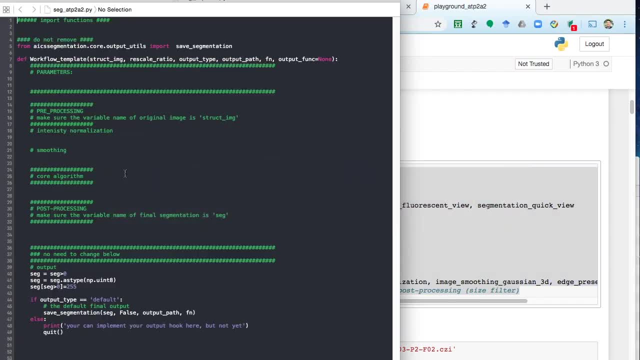 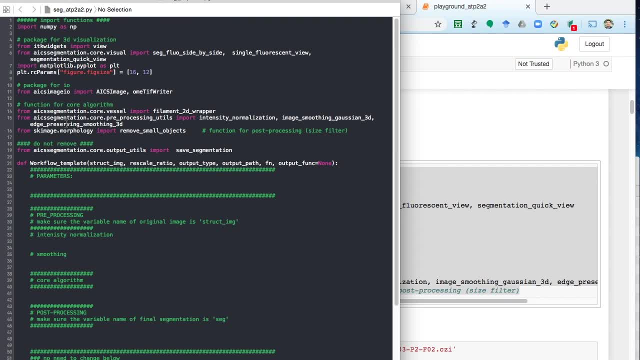 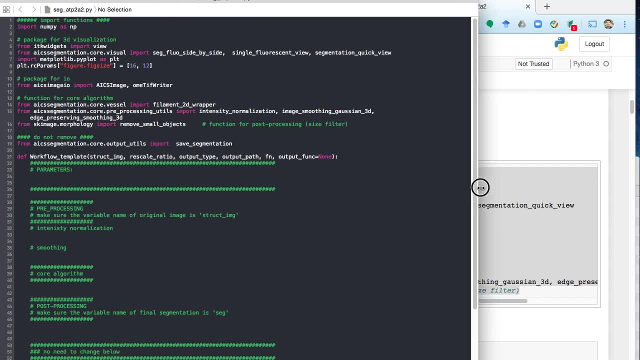 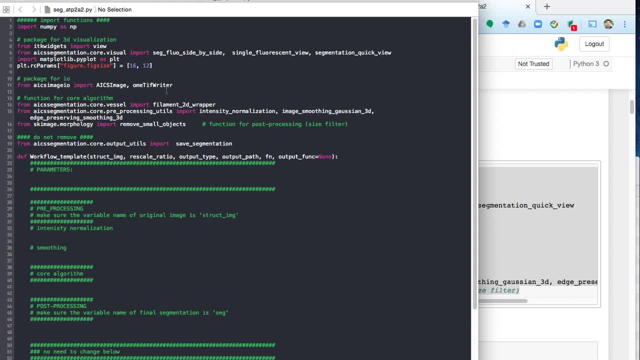 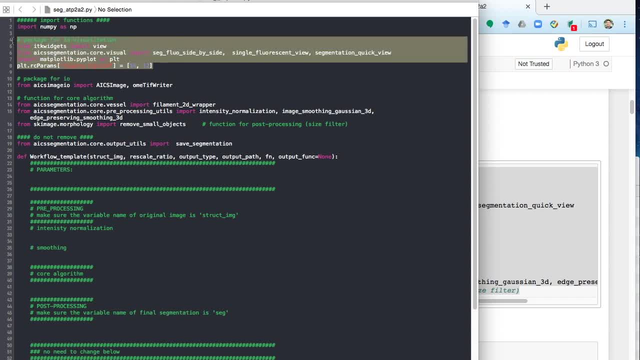 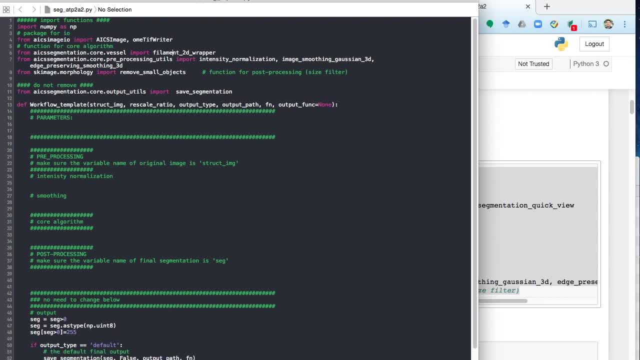 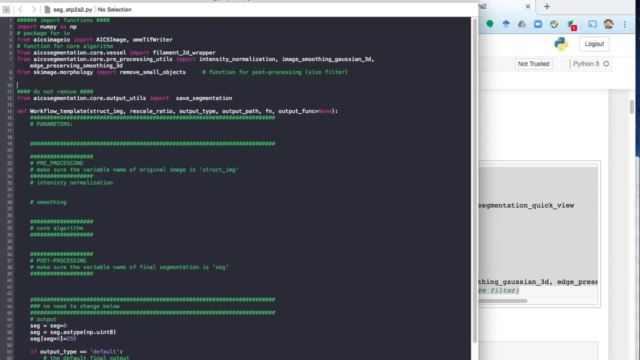 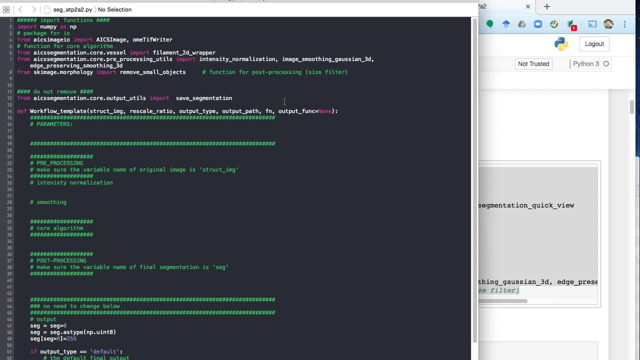 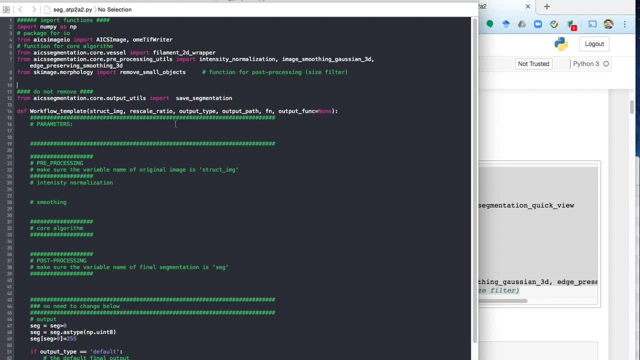 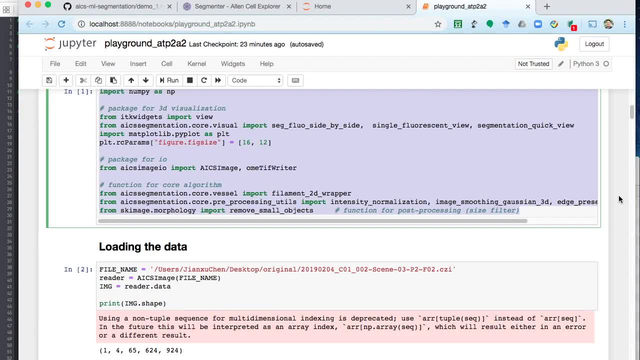 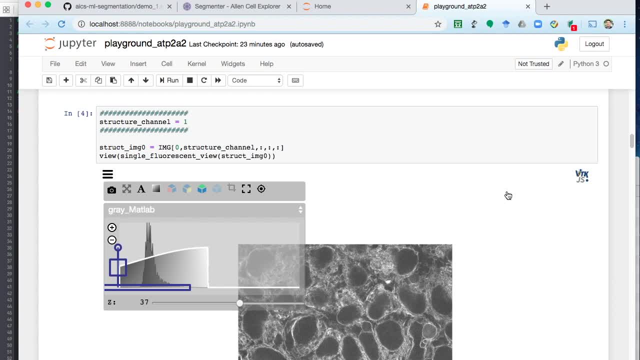 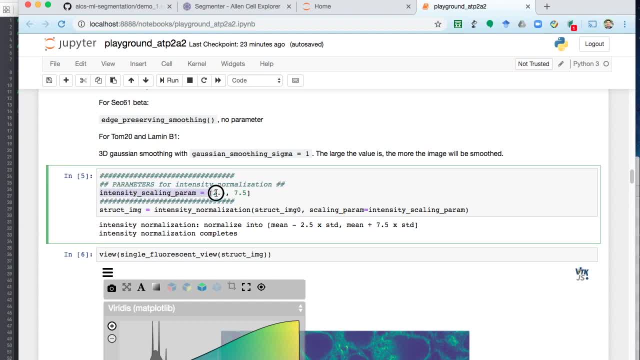 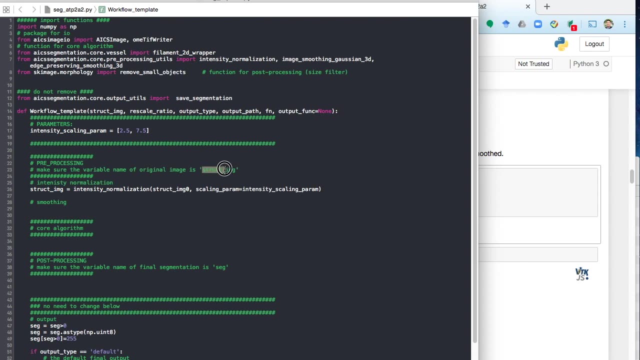 Here I have the parameters for preprocessing. Then we can just copy and paste the functions step by step. Then we can just copy and paste the functions step by step. Please keep in mind that it's very important to double check the variable names. 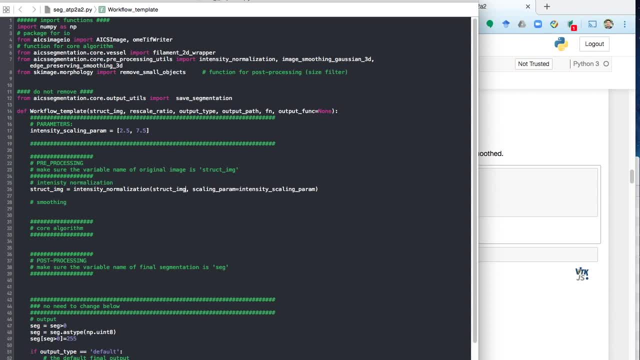 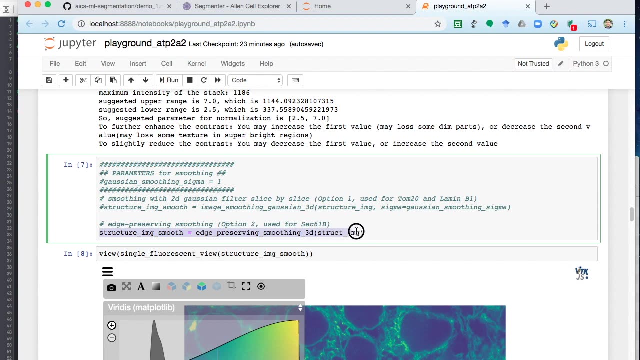 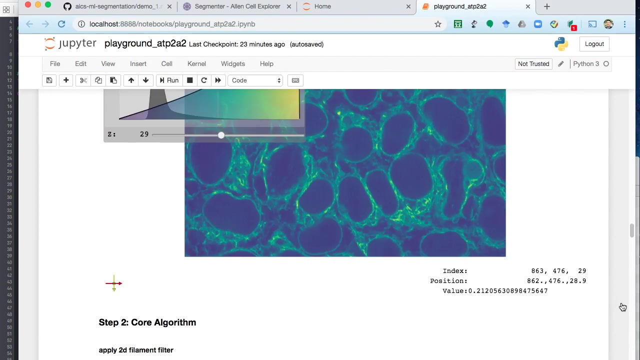 Please keep in mind that it's very important to double check the variable names. as emphasized in the template, The variable inputs for preprocessing should be structured: The variable inputs for preprocessing should be structured under UPCA1- point-vertical-ugn. Keep going, and here we'll copy the function for smoothing. 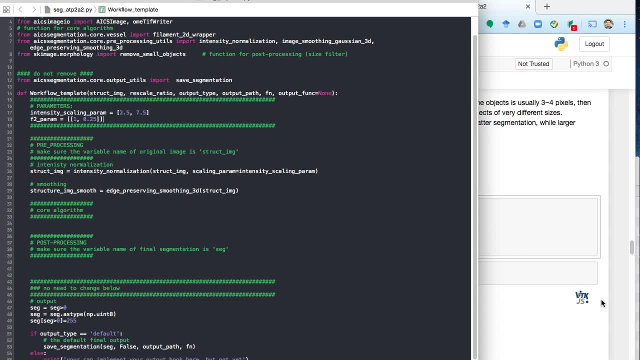 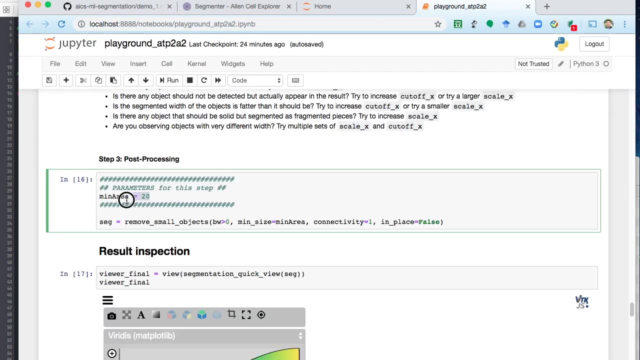 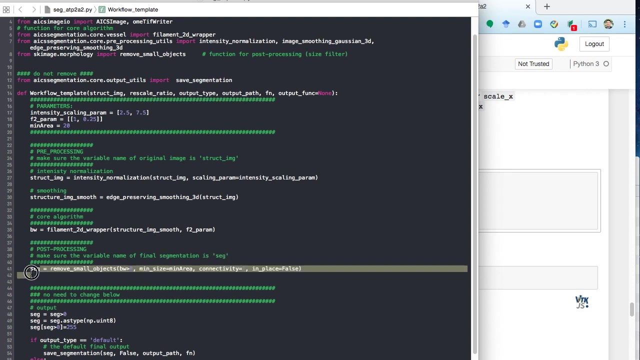 We'll have the parameters for the core algorithm and the function for core algorithm. Last, we'll copy and paste the parameters and the function used for post-processing. The variable name for final segmentation: It should be seg. Remember that you also need to change the function name here. 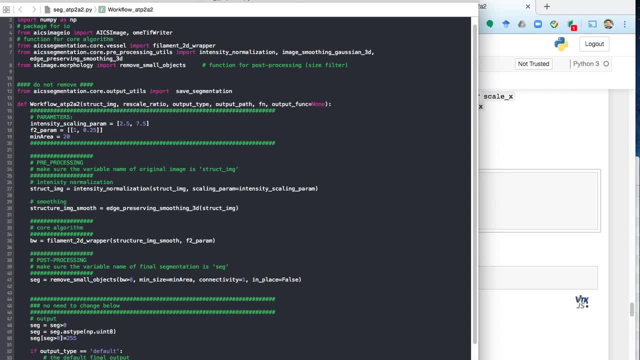 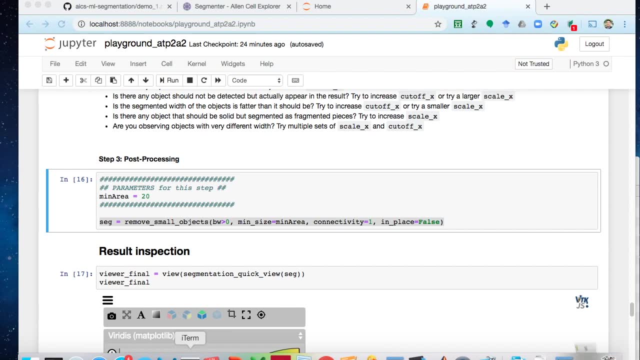 It should match the second part of the file name and will be used as the workflow name in batch processing. Once you're done and saved the Python file, you can run it in terminal. We'll open a new terminal window and activate the conda environment again. 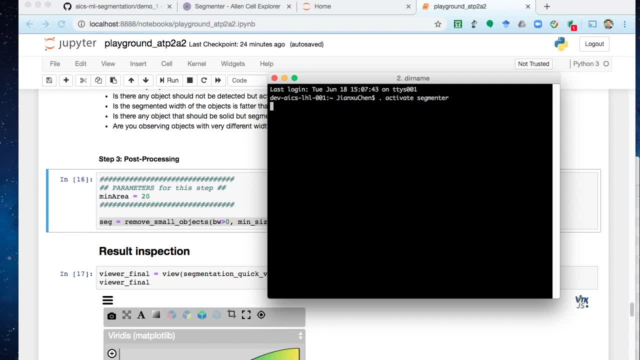 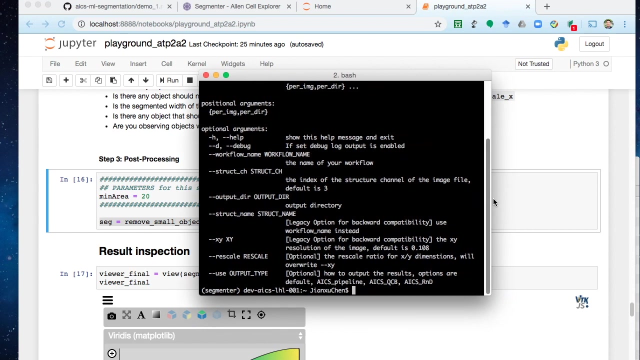 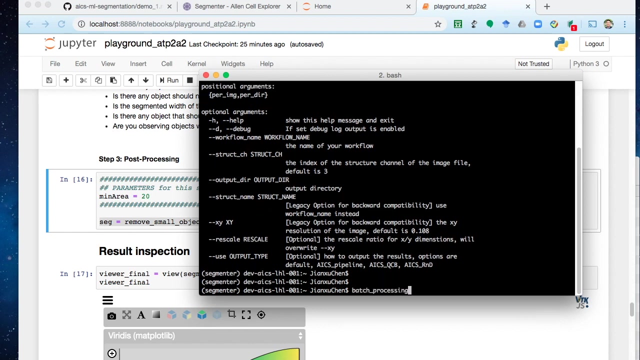 The command line for doing batch processing is very simple, but you can always get help by typing batch__processing-h if needed. Nice, Great, Awesome, Great. To batch process images. start with batch underscore processing and specify the workflow name, in our case, ATP282.. 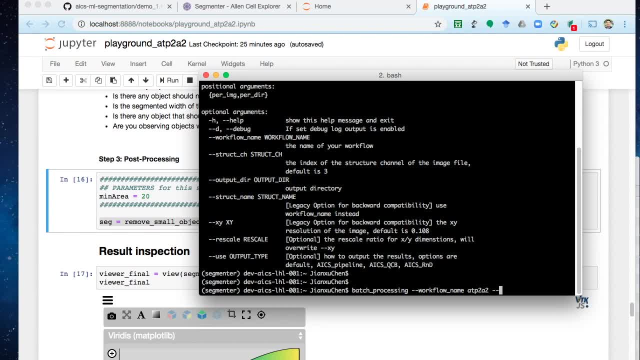 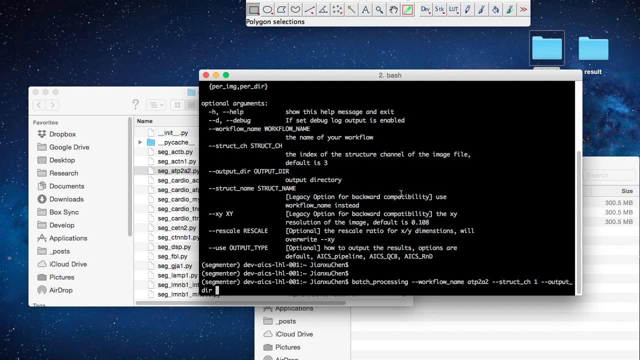 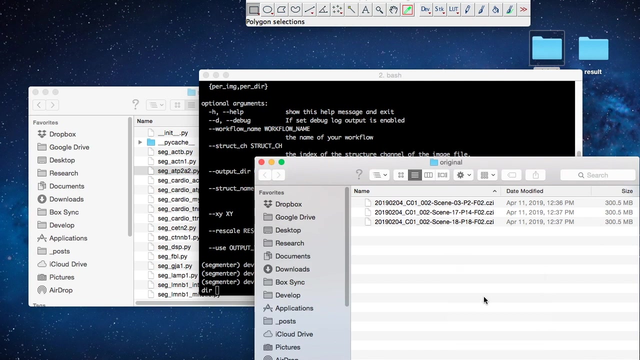 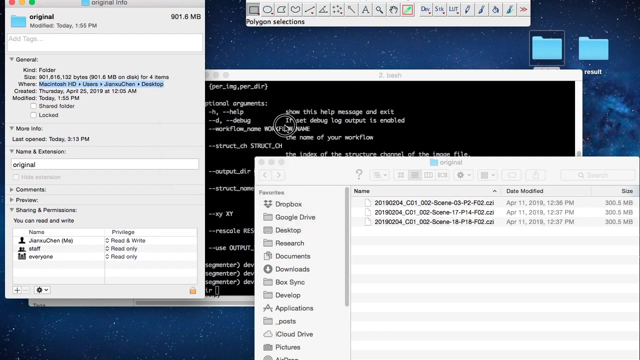 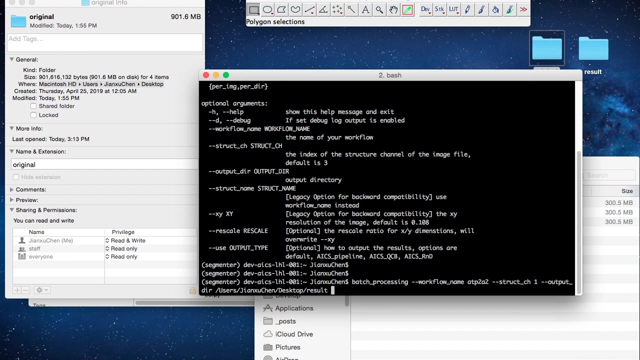 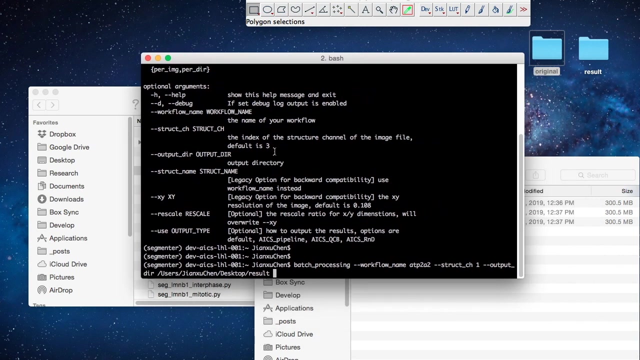 The index of the structure channel in our case is 1, and where you want to save your results, You can just copy and paste the folder name here. We want to also specify to do it in a per directory mode as well as the input directory. 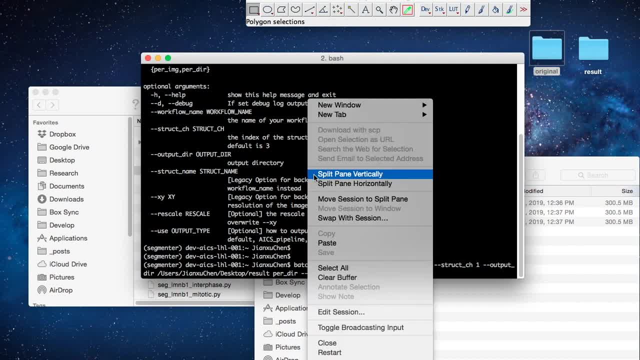 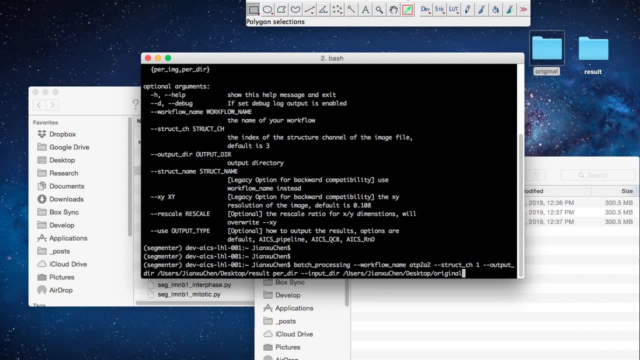 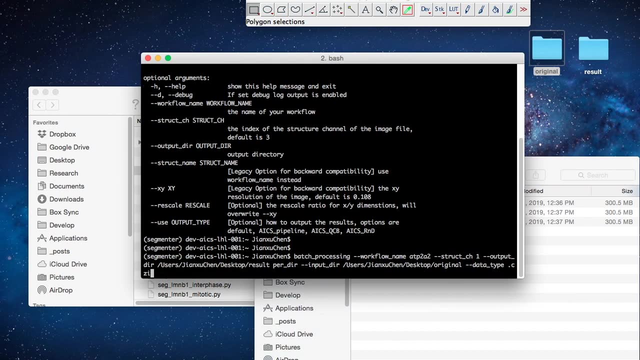 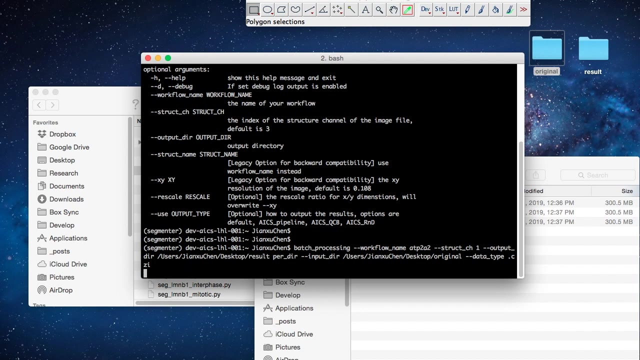 We'll again copy and paste the file path here. We also need to tell the program that we're looking for all the CZI images in that directory. Now we're ready to batch process the images. Usually it can take about 30 to 60 seconds, depending on the size of your images. 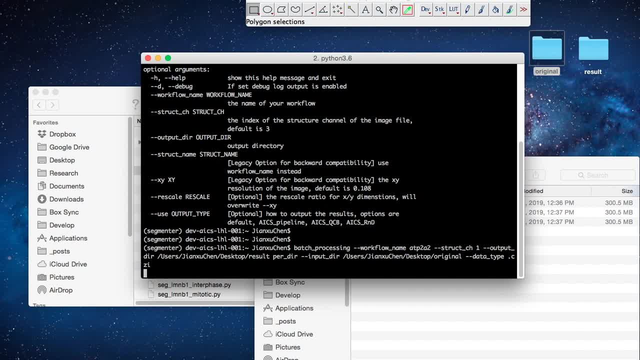 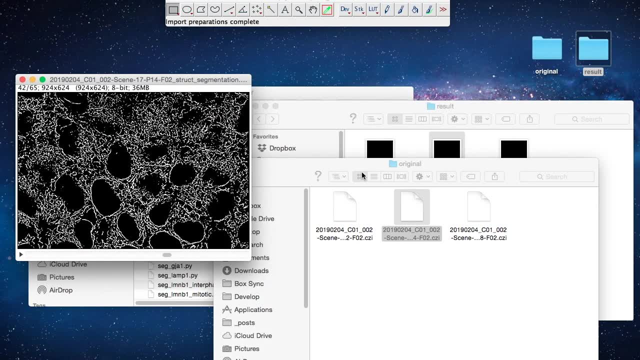 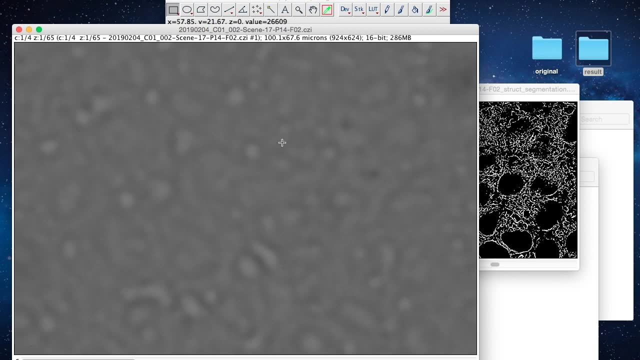 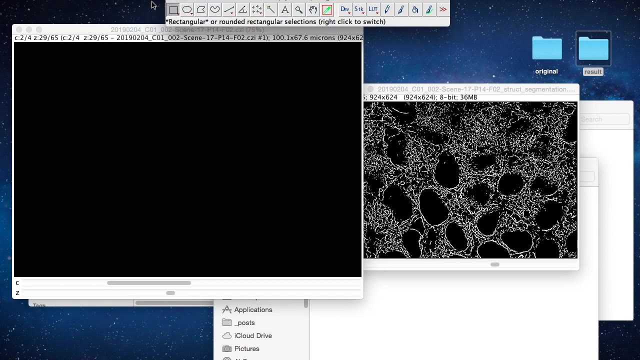 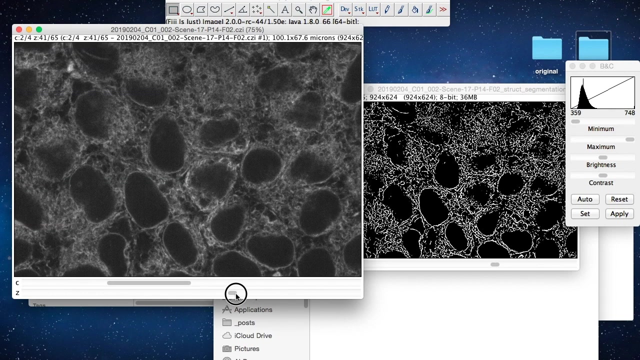 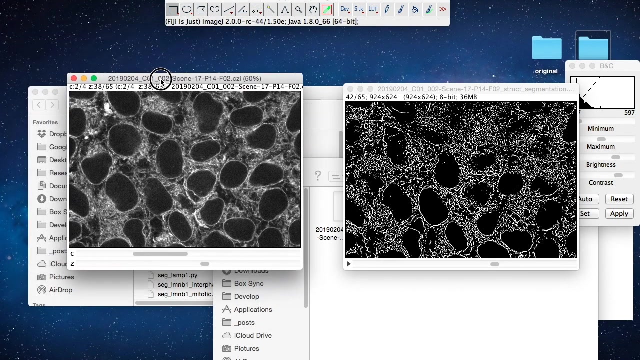 For demoing purpose. we fast forwarded the video a little bit to show you the results. We're opening one pair of original image and segmentation to compare them. Let's start with the original image. Now we have the original image and the segmentation result side by side.